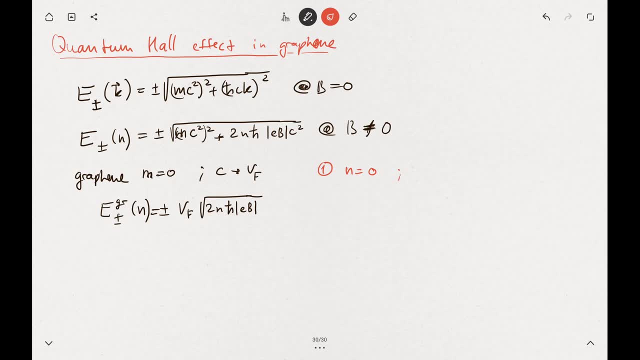 So when you have a zero Slendau levels, the index equals zero. the energy is also equals zero. So when you have a zero Slendau levels, the index equals zero, the energy is also equals zero. And that's quite different. That's very different from the two-dimensional electron gas. 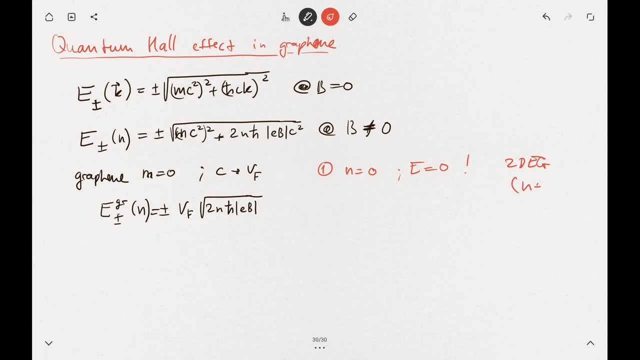 When you have N plus one half bit, because of the simple harmonic oscillation problem. So it's not zero energy for zero Slendau level. In graphene, the zero Slendau level has zero energy. Then the second one is that energy of the Slendau level. 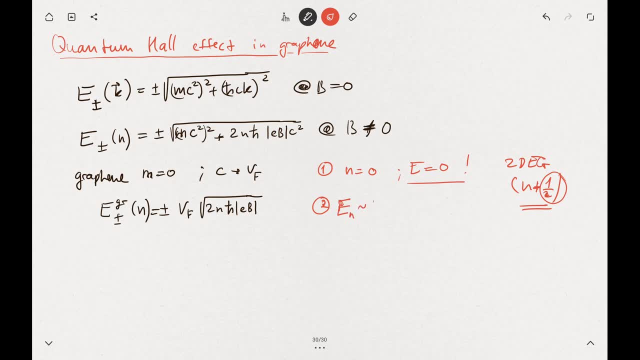 is proportional to the energy of the momentum of the SO начинаем giant scale to the square root of B in graphene and in the 2-DEG it's proportional to B, that's in two-dimensional electron gas, and the other one is that energy is also. 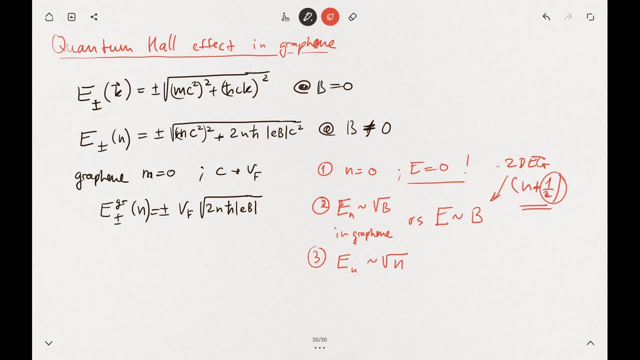 the energy of Landau level is proportional to the square root of the Landau level index, and in two-dimensional electron gas it's proportional just to the Landau level index. then the last bit is that the degeneracy is different. the degeneracy is also different because in graphene 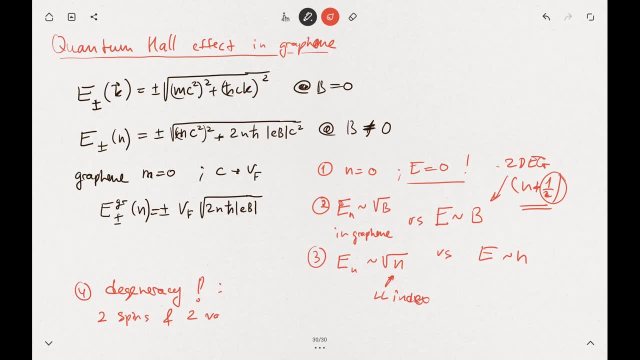 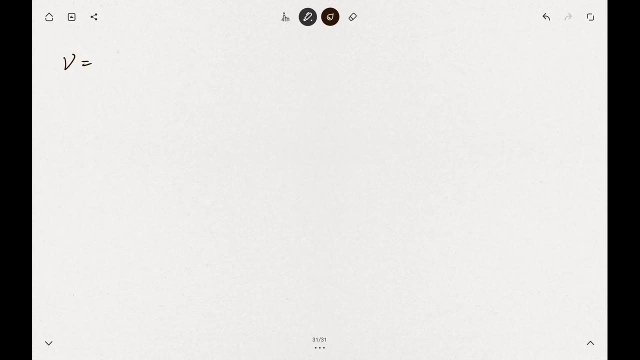 you have two spins and two valleys, so it's a four-fold degeneracy. you have two spins and two valleys, so it's a four-fold degeneracy. now we can write down this in terms of the degeneracy. so the filling factor is carrier density times H over EB and the Landau level, so at n equals zero you. 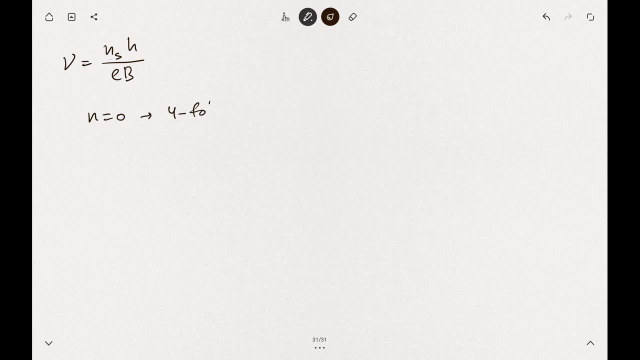 will have a four-fold degenerate and zeros Landau level and it's centered, centered at E equals zero and that means also NS equals zero. so the carrier density is zero and it has to be separated by the filling factors of her plus and minus, minus two, four, in order for it to be symmetric. so we can draw this on the 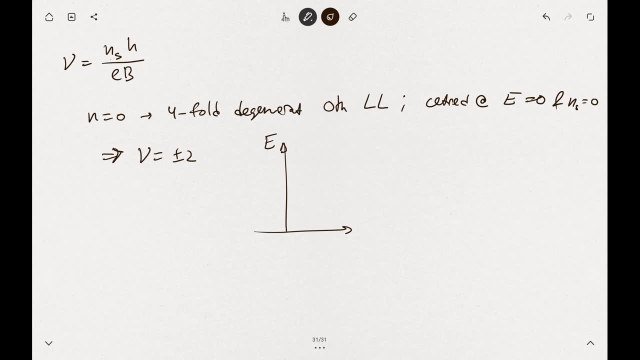 energy scale. this will be our use. G then still states: and this is, let's use this one to be zero, so there will be. there will be the energy level. so the zeros landau level is zero and this is gonna not be equal negative zero, so it is gonna be. 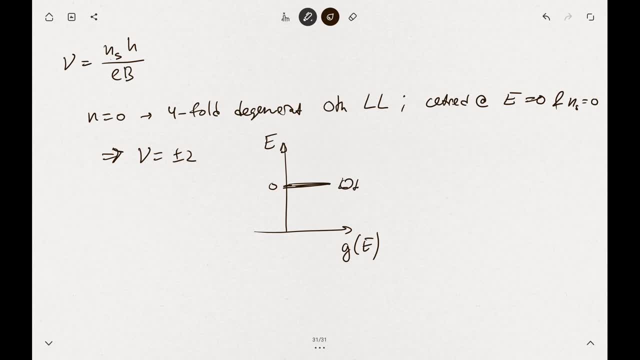 6. nee, It's not even equal zero, but it's zero. I don't know its because it's a eureka. it's coming into the space, it's going to be linear, so let's do this 0th Landau level, and then we have some other Landau levels as well. so the first, second minus. 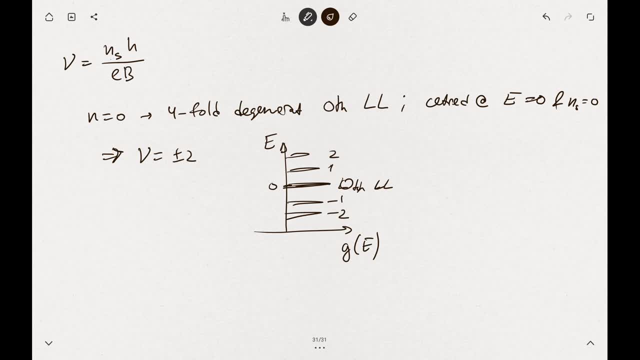 first minus second and so on. but when you draw them on the carrier density scale, so using this NS, the 0th Landau level would would actually be separated by this plus minus two degeneracies. so if we have, this is our filling factors, which is kind of proportional to the density of states. 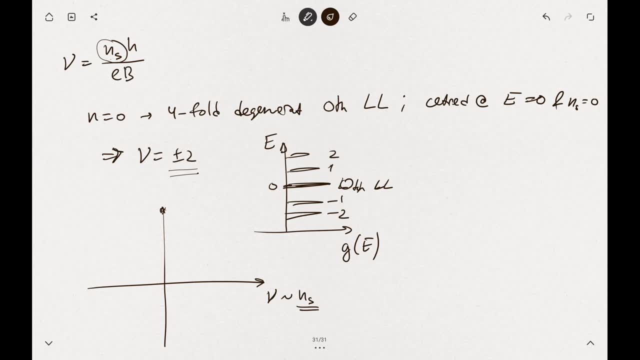 to to carry density, and this is, for example, Rho xy, just to see the quantization, but use Sigma xy because that's that's done, equidistant. so around the filling factors plus minus two you have the plateaus in the conductive, in the Hogan, in the 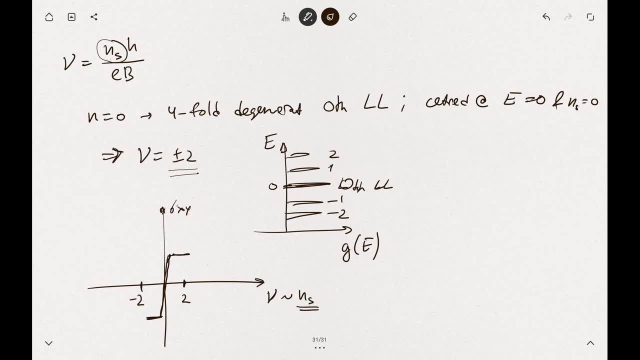 Sigma xy and these plateaus will be one half of four e square over H. that's a general unit because you have four fault degeneracy. so it's four e square over H and it will be half half integer. basically, in this case you will have minus one half four e square over H for this state then.